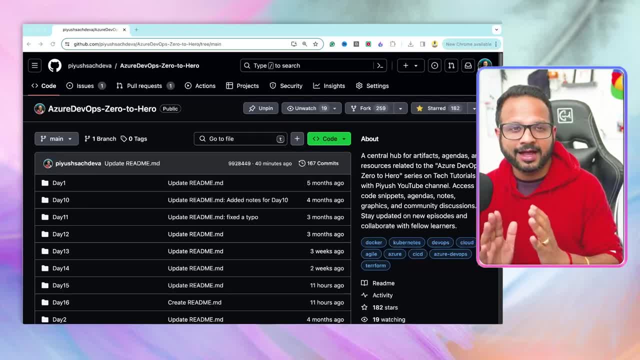 with this video, Else, I would highly recommend going back and have a look at all the videos and do the actual hands-on and then come back to this video later on. This should be referred as the last handouts, So I'm in my GitHub repository and you should already have the link by now. If not, you know. 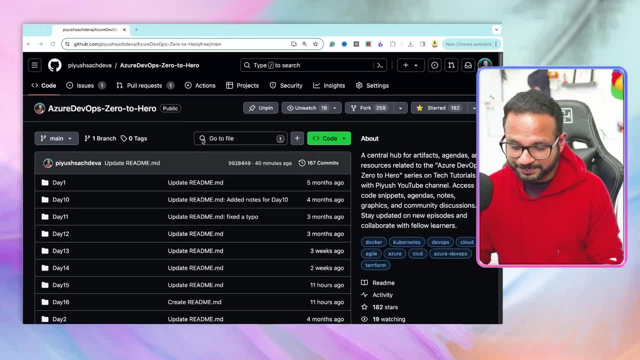 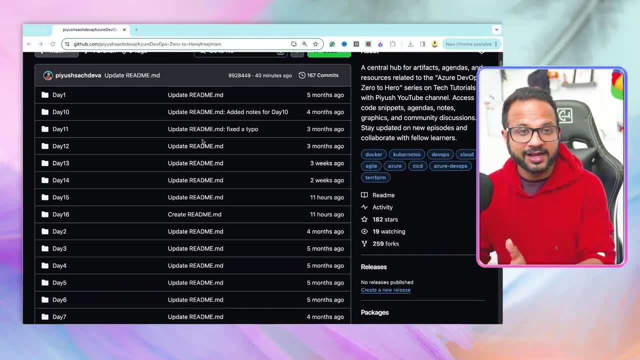 where to find it. It'll be there in the description section as well And, as we have seen, for every video there is a dedicated folder for it, And in that folder I have provided all the screenshots, all the diagrams, all the notes, all the code snippets and everything that you need. So, for 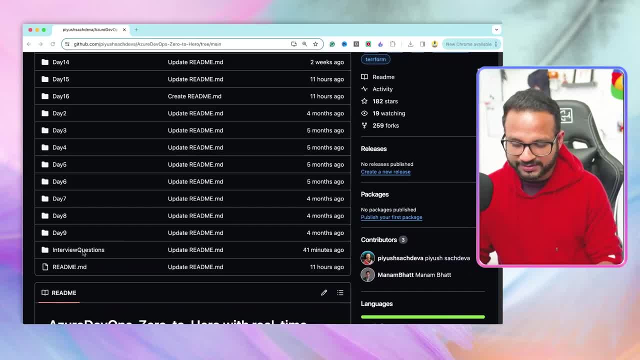 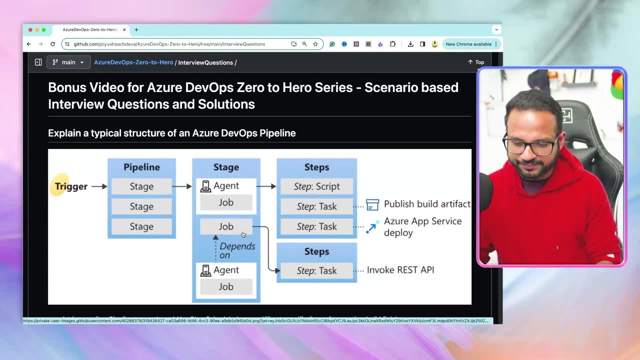 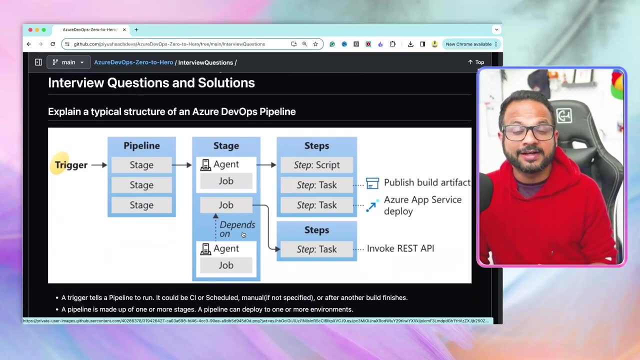 this particular video. I have created a separate folder which says interview questions. You go inside that and there'll be a readme file. We'll start with the first one. The first question is: explain a typical structure of an Azure DevOps EML pipeline, right? So if the interviewer asks: 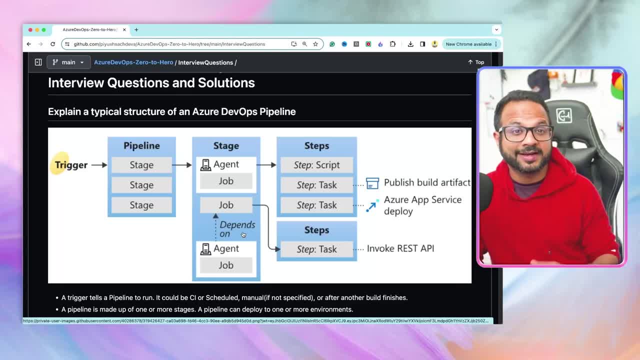 you that question. that means they are asking you or they are expecting you to explain the overall structure of that EML pipeline. So it will start with trigger, This trigger. it could be anything, It could be a scheduled trigger, or it could be a manual trigger, or it. 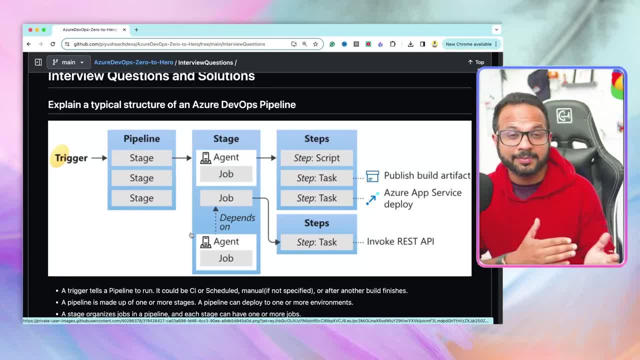 could be you know something that's been triggered by another pipeline. or it could be a scheduled trigger, like: run this pipeline at a certain time at a certain day, Right? So trigger defines how this pipeline will be executed. If there is nothing, that means it is a manual trigger. 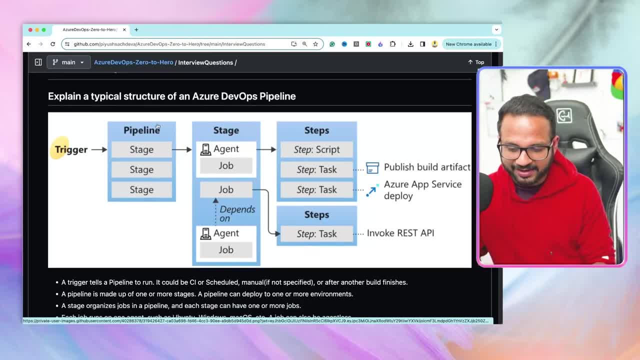 Right. So that is trigger. And then we have a section called pipeline and this pipeline is divided into two sections. So this is the pipeline and this is the pipeline. So this is the pipeline into many different steps. So the first is stages. So there are different stages. 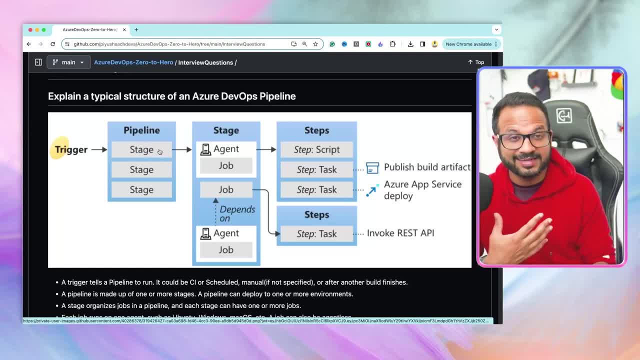 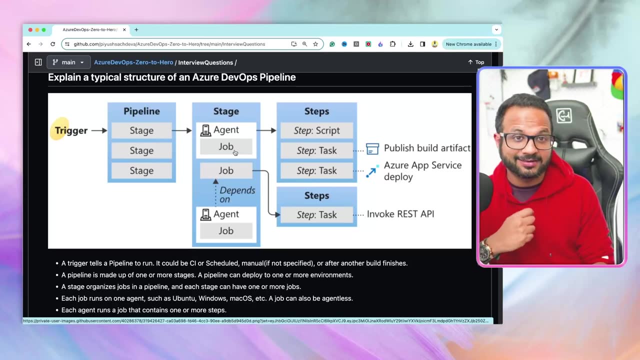 different stages for build, deploy, test and so on, And then each stage is divided into multiple jobs. Jobs is something that would run on an agent right, So each stage can have one or more jobs right And these jobs it can run on agent or it can be agent-less, Like certain tasks does. 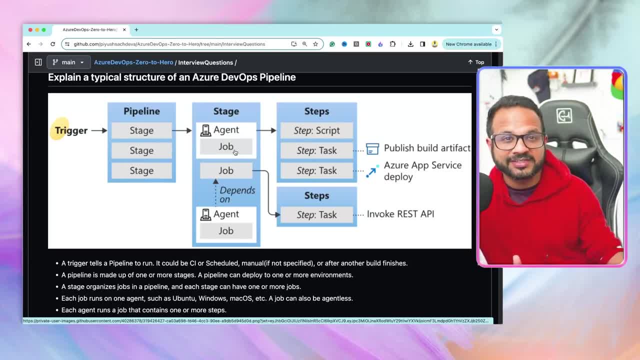 not require agent. For example, you are running just an arbitrary script like, let's say, copy command- copy this file to this directory, right? So it does not need an agent. So you can run that on agent-less fashion as well, Right, And these jobs. 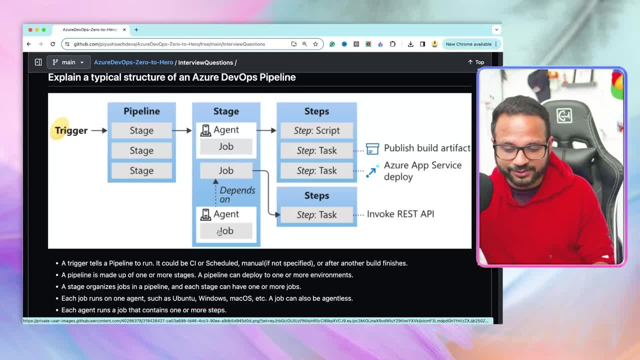 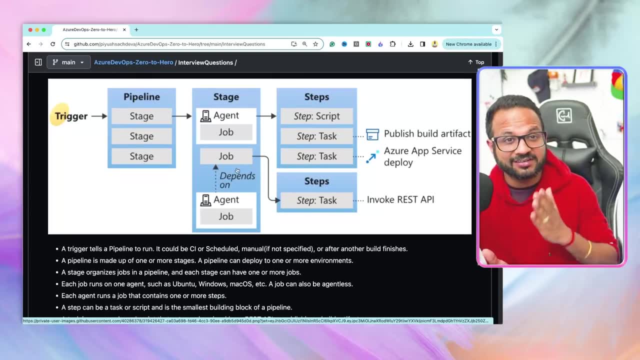 can be dependent on each other. Yes, like execute this job once the previous job is completed, and so on. And actually what happens is agent run a job And in that job you have multiple steps. These steps could be a script or a task right Scripts such as, you know, a shell script. 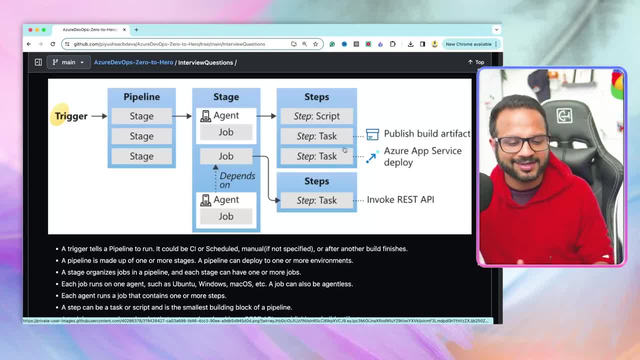 a bash script or a power shell. that could be a script, A task, such as publish, build artifact or Azure app, deploy or invoke REST API. So these are the tasks. So, if we go from bottom to up, the smallest unit is a step. okay, Step could be a task or it could be a script. 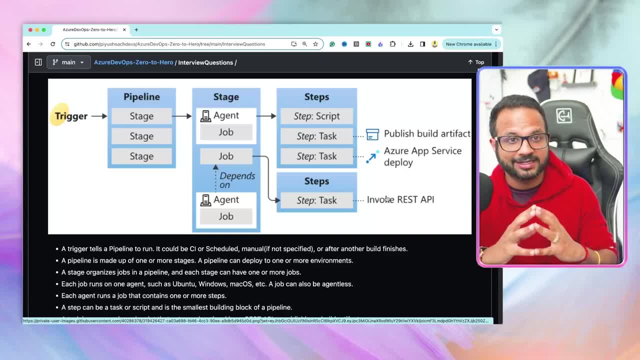 or collection of multiple steps, is a job. Job runs on an agent. you can have multiple jobs in a stage and a pipeline can have multiple stages. So this is how they are tied together. This is the hierarchy of an Azure DevOps- YAML. 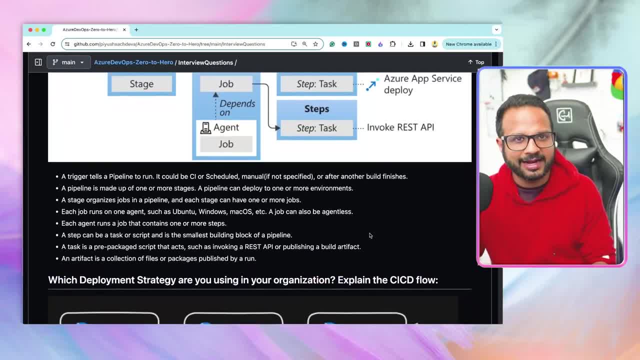 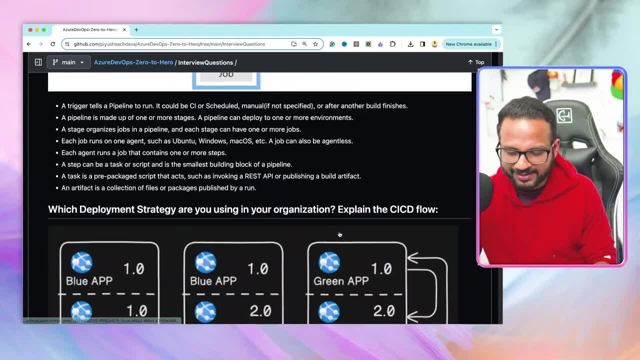 pipeline right. So have a look at that, And if you have implemented it- you have already seen it, you have already created it- then there shouldn't be any issues, right. The next is: which deployment strategy are you familiar with? Explain the CI-CD flow right. 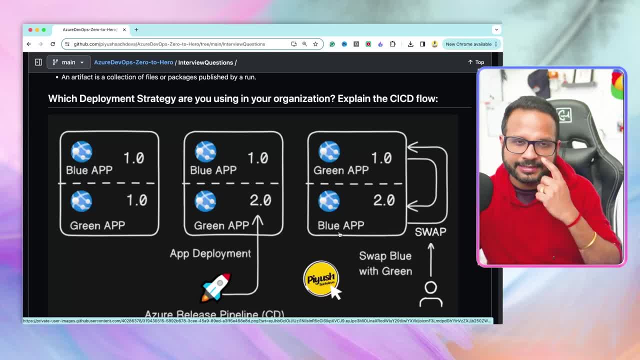 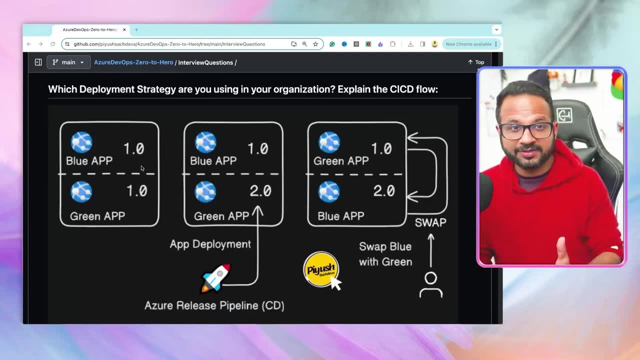 Blue-green and rolling update are the most common deployment strategies And in this example we'll be looking into blue-green. So what exactly is blue-green? Let's have a look, all right. So how it works is, let's say we have an app running version 1.0. Let's call this a blue app. 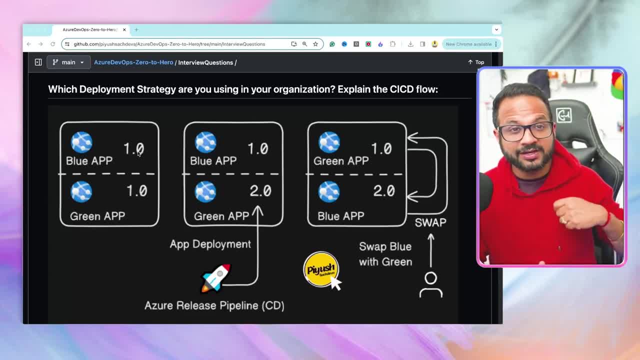 So this is the blue version of the app. What we'll do? we'll create another app with the same application code, with the same version, and we'll call it a green version of the app, but this will also be running version 1.0.. Now we'll do. 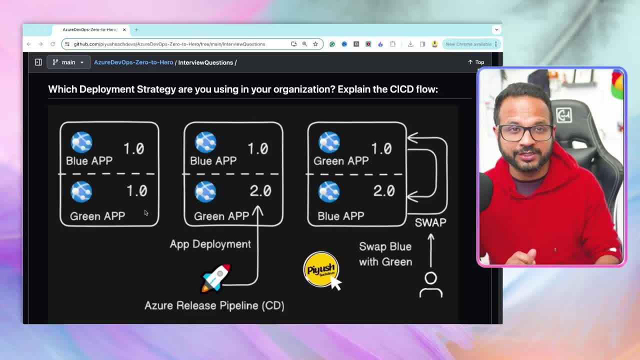 everything on the green app, the newer app that we just provisioned. So we'll do the build, we'll do the testing and then we'll do the code deployment. Everything will be on the green app. So now the green app has the updated version, updated production code, which is not yet. 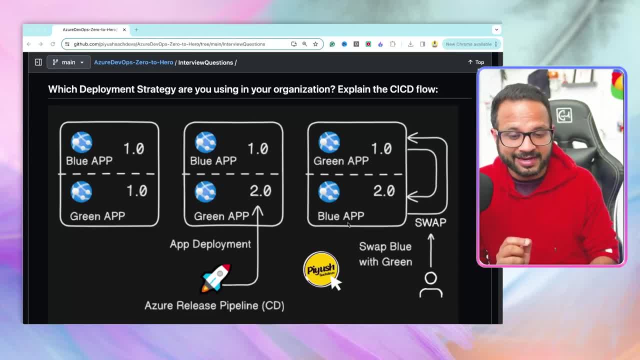 live for the viewers. So before making it live, we'll do a swap Now. once we have done the swap now, our green app will become 1.0 and our blue app will become 2.0. So we did not touch our. 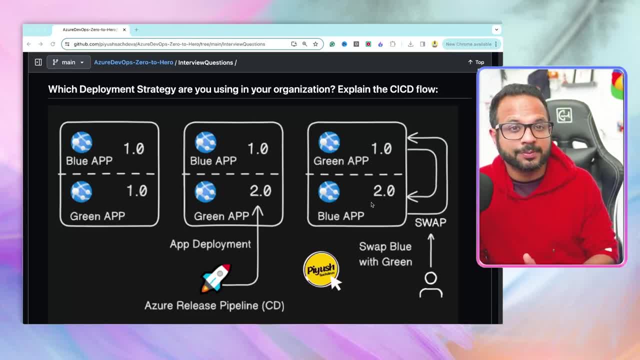 live production environment before the code was deployed to the environment. So this is what we did, And there is no downtime, There is no user impact. Once everything is done, only then we made the switch. Now the users will be redirected from the version 1.0 to the version 2.0, and we can. 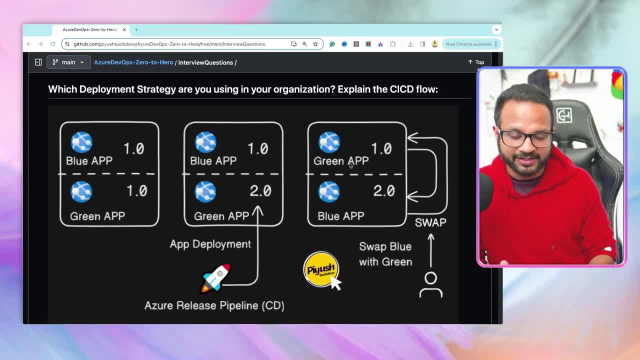 then destroy this green app version 1.0, right. So that is how our blue app 1.0 become blue app 2.0. With minimal impact, with minimum downtime or in fact, no downtime. it's just a DNS swap in this. 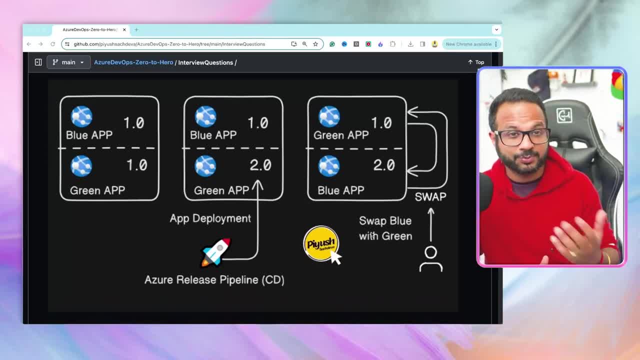 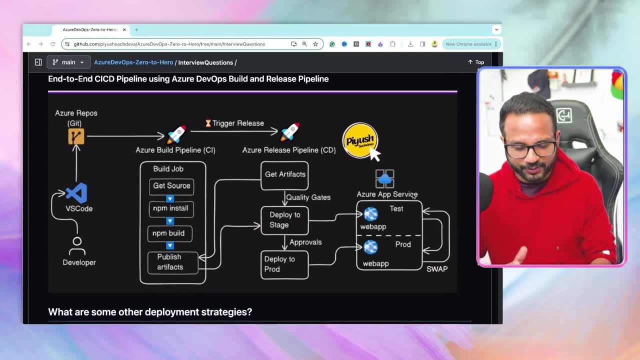 case, And this is how blue green works. After you have explained what a blue green deployment is, the next part of this question was explain the CICD flow right, So this is what you can explain. This is the diagram from one of the videos in which a developer, or multiple developers- 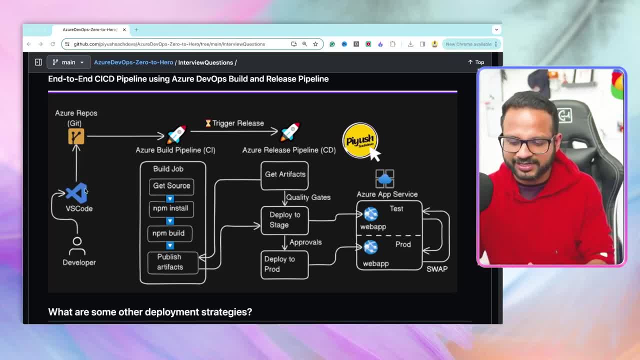 commit the code with the help of ID such as VS Code, And once the pull request is approved and merged, a build is triggered. That build will do certain steps, like download the source code, install binaries and dependencies, run npm, build and then publish. 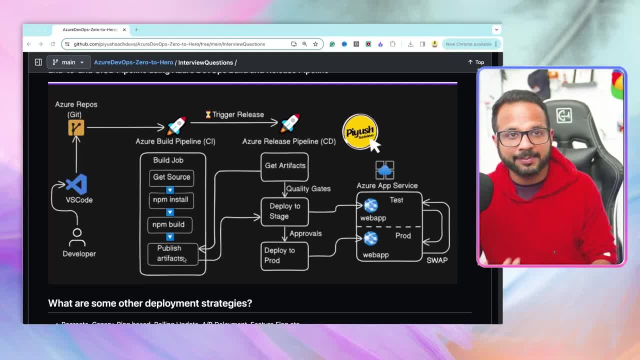 the artifacts. These artifacts will be published to the pipeline location and as your CD pipeline. then get the artifacts from the drop location or wherever the location we have specified and it will deploy to the stage. In this case we have additional quality gates before the deployment, such as if all the test. 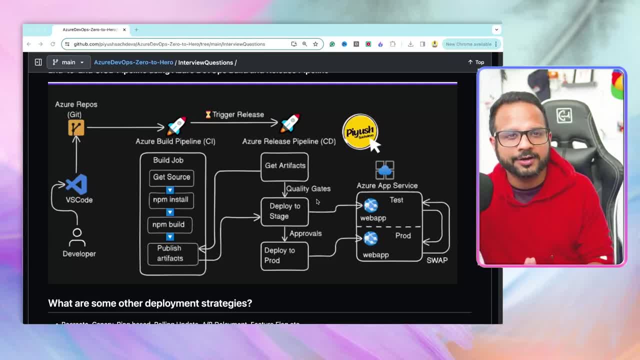 cases passed, only then do the deployment. or we can add manual approval as well. So if it is approved by one or more approvers, only then the deployment will be triggered, and so on. There are different quality gates that we have discussed. right, So that deployment happened and then it 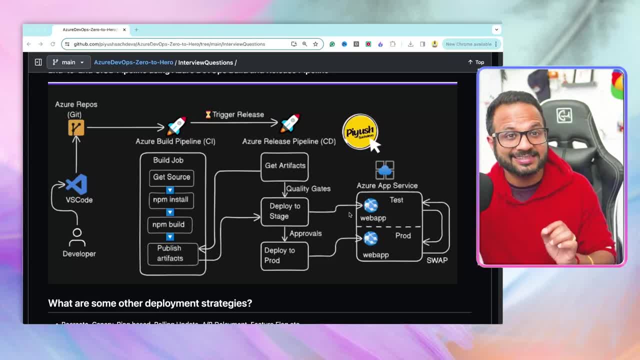 should be deployed to stage right. Stage in this case is the deployment slot when it comes to web service. So we have deployed to that slot And once we have got the approval for deployment into production, then we deploy it to the production slot right And based on that, like if you are, 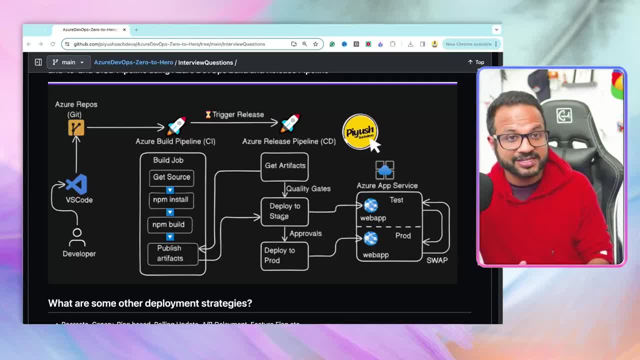 using blue green, then you can have only one stage over here or a step to swap between staging and production. If that is not the case, you can explain like either of these two scenarios: Either you have one stage and multiple slots or you can have 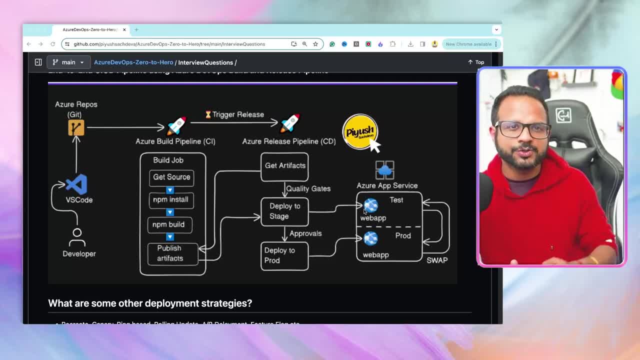 multiple stage and one slot right. Either one is to two or two is to one. It depends on the use case. It depends how you are more comfortable explaining it, right? But I've explained blue, green and the same strategy you can use over here Now, once you have explained that there could be. 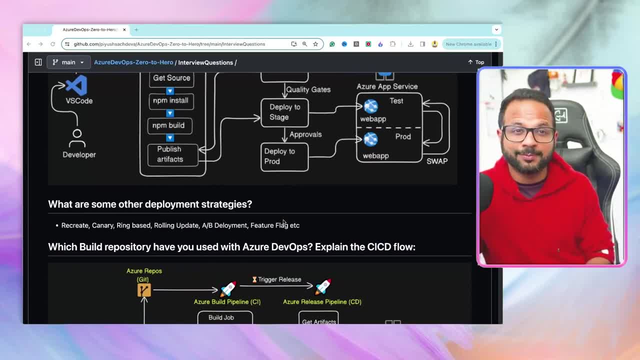 some additional questions like: okay, now you have explained blue green deployment, What are some of the other deployment strategies? Then you can explain. there are different other strategies, such as recreate, canary ring based, rolling, update, AB deployment, feature flag and so on. So you can have a look, have a read on all these deployment. 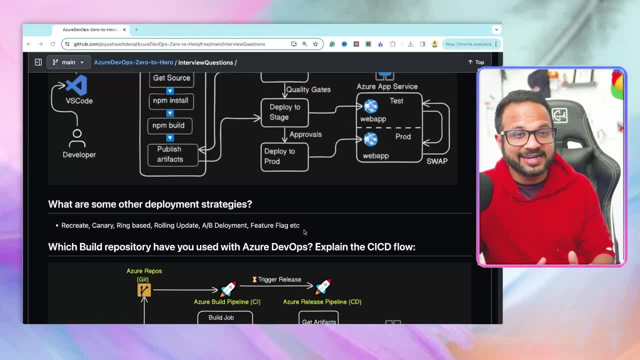 strategies as well. If you want, I can create a separate dedicated video for discussing all the deployment strategies. So let me know if you want me to do that. Let's just read about it. It's pretty straightforward, It's pretty simple. Just like we have blue, green or like these are other 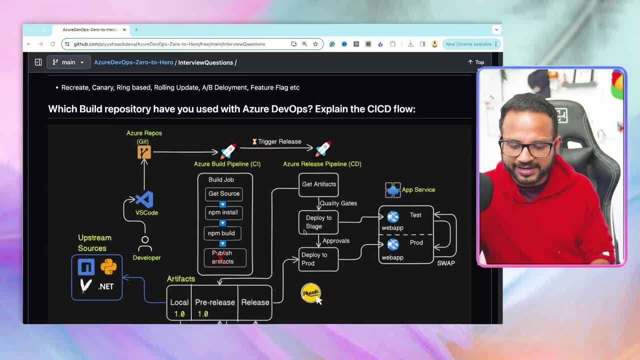 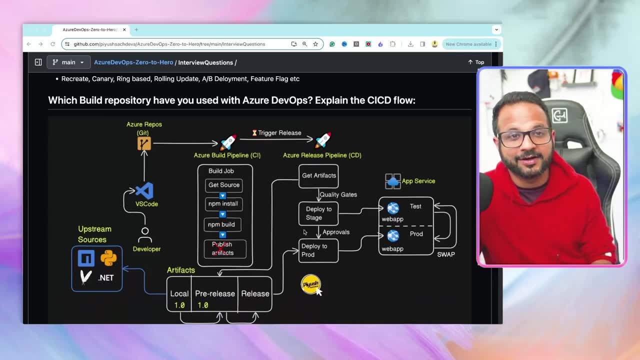 deployment strategies. Now the next question could be: which build repository have you used with Azure DevOps? So let's say, if you have a Docker based build, so you might have used Azure container registry. If it is, you know, a zip file, tar file, npm build or any other artifact you can. 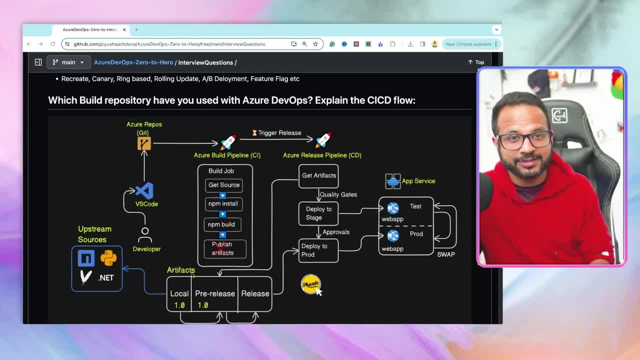 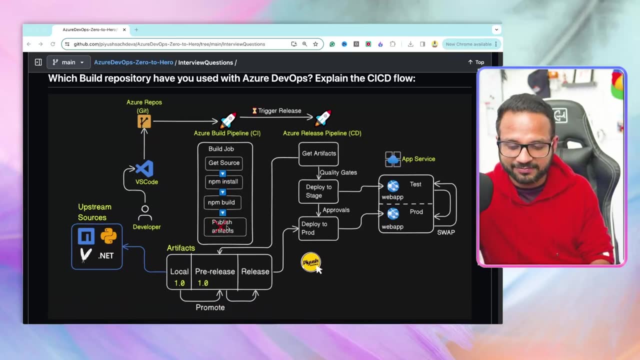 also use an inbuilt repository within Azure DevOps which is called artifacts. So you can explain this entire flow. Again, this was part of one of the video And you can have a look and you can explain this entire flow. Instead of publishing the artifact to the pipeline itself, the Azure CI pipeline, publish it to the 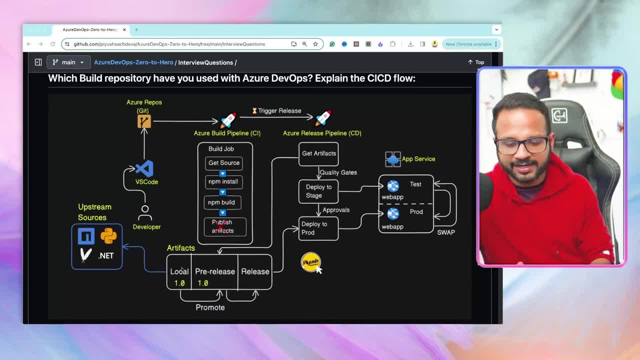 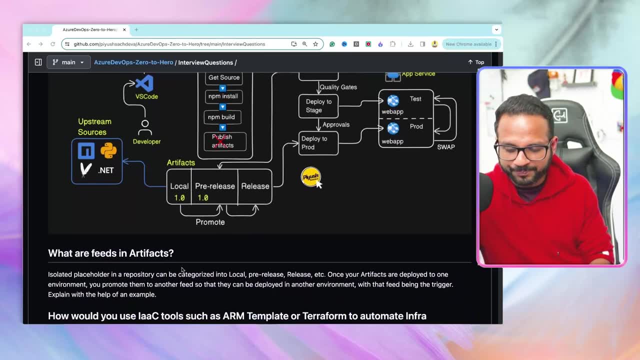 artifact, So by default it goes to the local feed And then you can promote between one feed to another and finally deploy it to the environment. Now the question could be- there could be some follow up questions like: what are feeds in artifacts? So you have explained feeds to us. 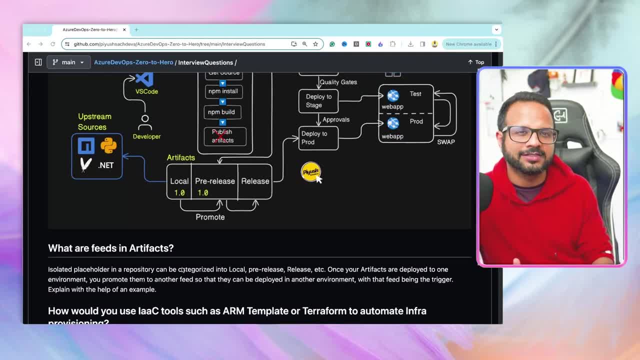 Now, what exactly are these feeds And what is the use case of it? So you can explain: like when a build is created, it gets deployed to a local feed. So these are nothing but the isolated container within our artifact repository, And it is there to keep your build separate between 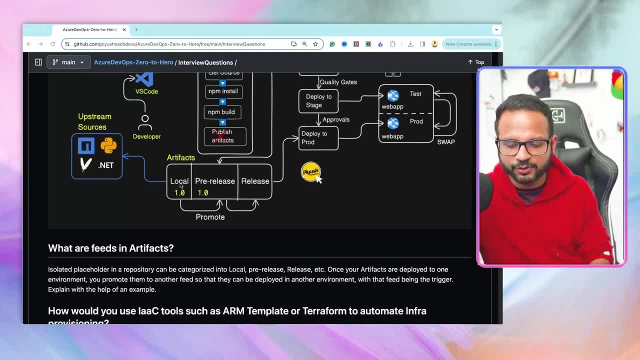 environments like, for example, build just been created, so it will go to the local feed And once you are ready to deploy it into the staging environment, you promote it to the pre release feed Right And in a release pipeline there is a trigger which is watching this particular feed. 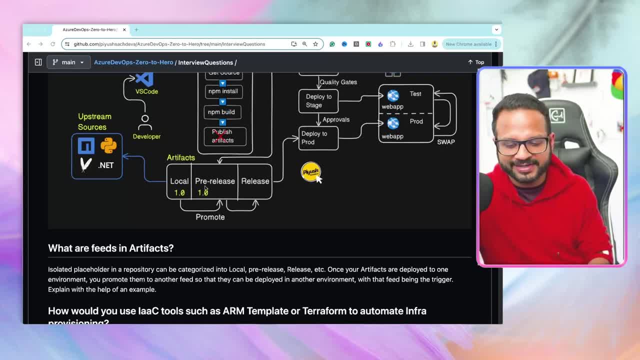 pre release. So if there is a package available in pre release feed, it will deploy that to the staging environment. Once it is deployed you can then promote the package from pre release to release feed And there is another stage in the release pipeline which is watching the release feed. And 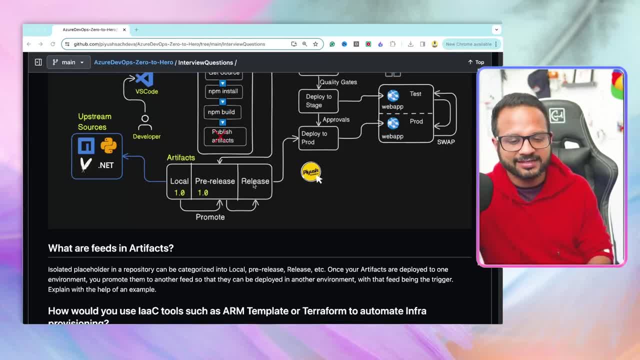 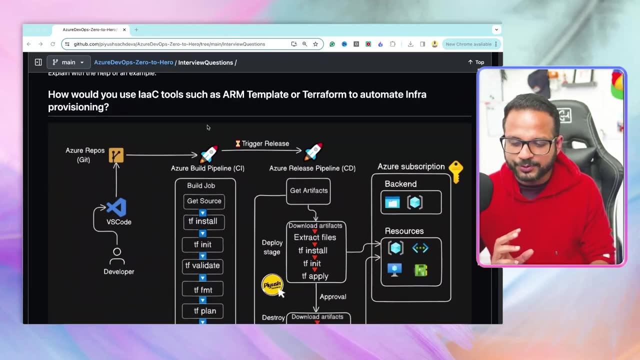 once the package is available in this release feed, then it will deploy it to the production environment And you can explain the quality gates and all other approval steps as well. So this is about Azure DevOps, artifacts and feeds. Now next question is: how would you use infrastructure as a code tool, such as ARM template or 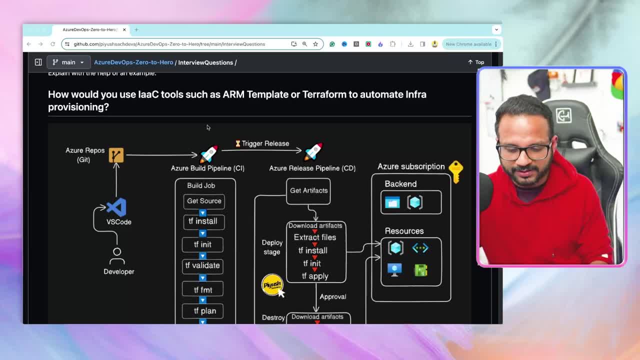 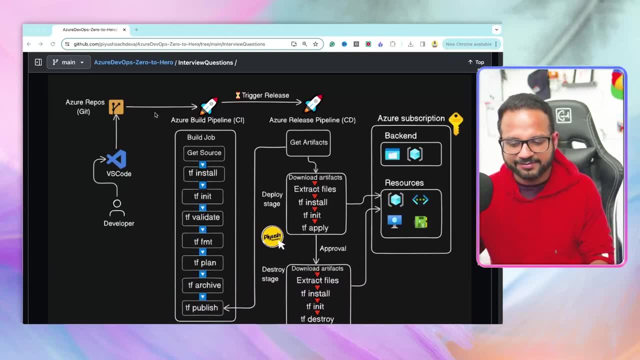 Terraform to automate infrastructure provisioning. This was part of video number eight, I believe right, and it has all the steps. again, the CI will be triggered once the code is merged And inside the Git repository or the Azure repos repository. 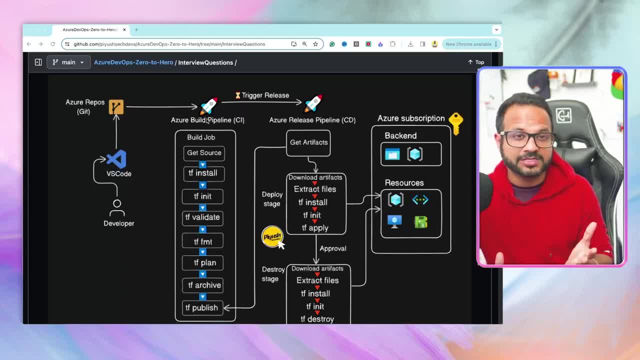 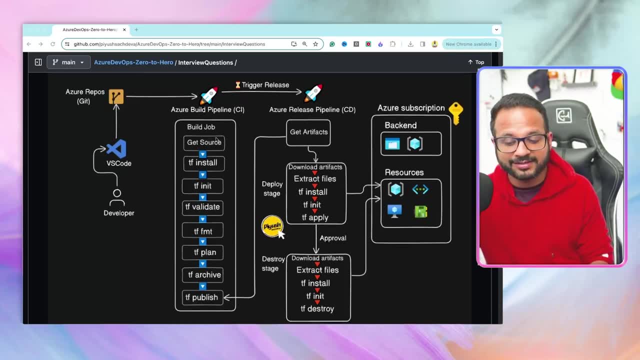 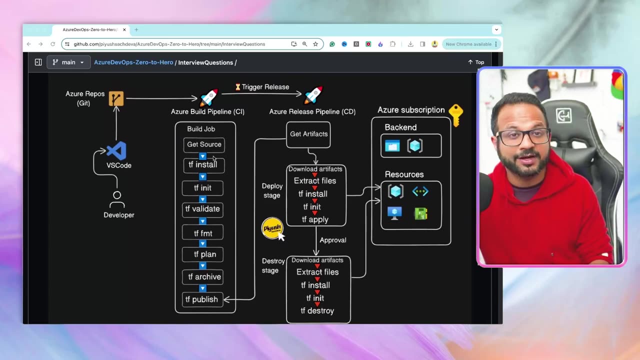 there will be Terraform configuration files, Or if we are using ARM template, then there'll be some template files And based on that, your first stage will be to get the source, like to download the checkout, the Git repository. then you run Terraform install because if you are using 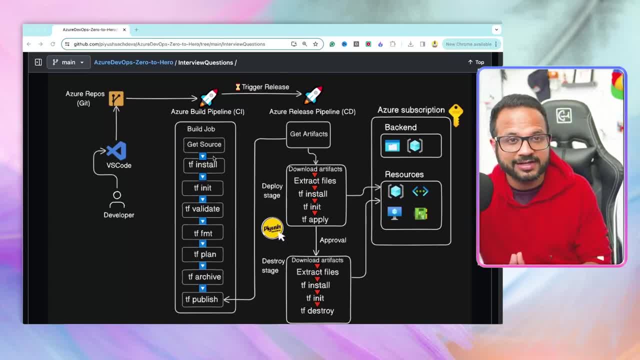 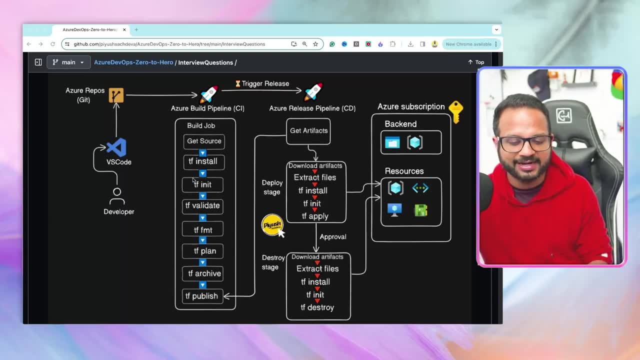 Microsoft hosted agent. the Terraform CLI might not be installed in that. So you will install Terraform And then you do Terraform initialization to initialize your back end. and to initialize because back end will be residing in storage bucket. it is a remote back end And it will. 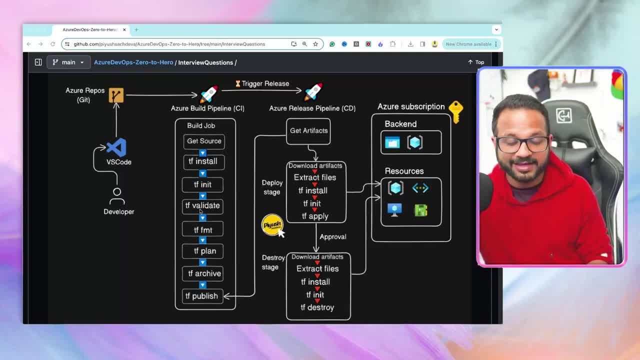 download all the dependencies and binaries, then you run TF validate or Terraform validate to make sure that your YAML is properly formatted And then you format it. if there is no syntax error, then you run Terraform plan, which will show you or which will, you know, give you a dry run result. 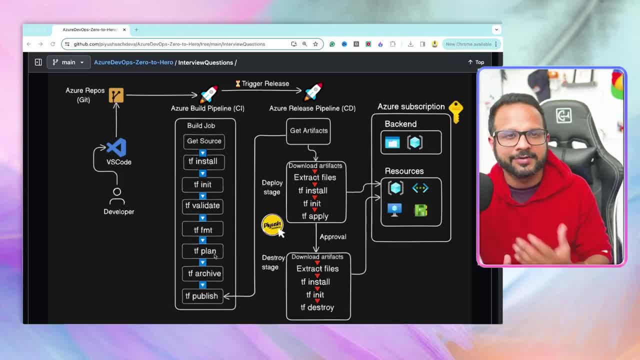 of how many resources will be created, updated or deleted Once you apply Terraform apply. then you do Terraform archive, which will package all the files inside a directory, inside a zip directory, and then publish it to be consumed later by the release pipeline, Right? So we've done that And 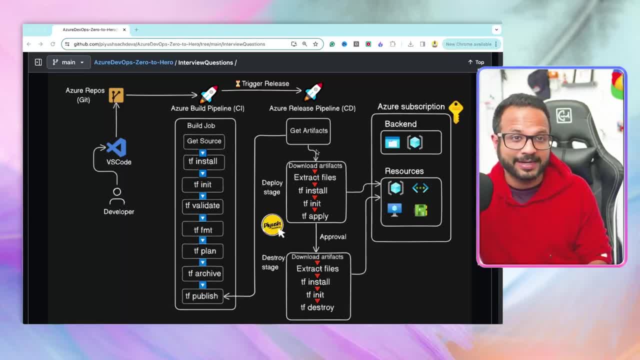 then, as your CD pipeline or the release pipeline will be triggered, it will download the artifacts, it will extract the file and it will do the Terraform install again. Why? again, because this is a separate agent. the build agent was separate and it was part of the Azure DevOps. 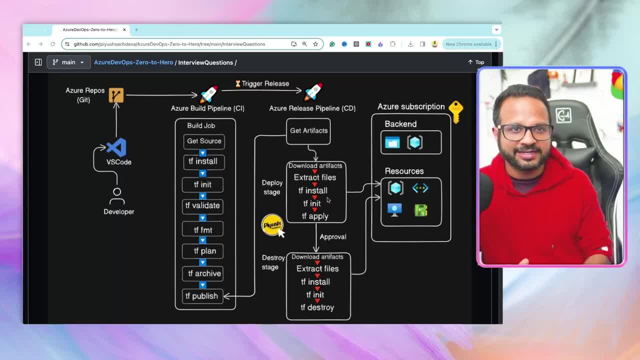 build pipeline. This is part of release pipeline. this is running a separate agent, a separate job. So that is why we have to install Terraform CLI again. then it will run Terraform initialization again to download the dependencies and then it will do the Terraform apply And then the 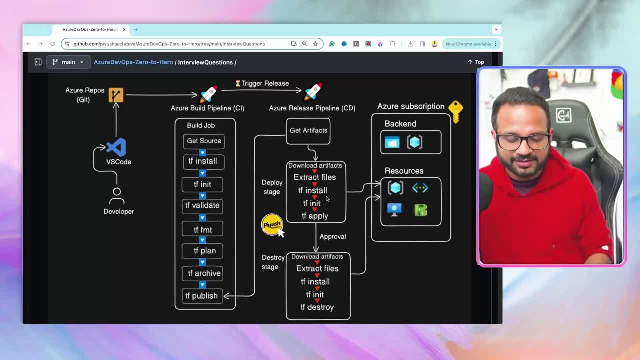 resources will be provisioned for the staging environment the same way, And and one more thing, so the resources will be provisioned in the Azure subscription with the help of service connection. Now you can have additional stage, or you can have an additional step to destroy all the resources. 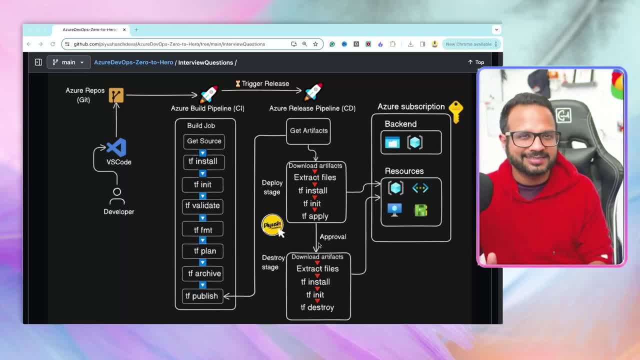 that were provisioned. So you can add a delay of, let's say, 30 days in between, or 20 days, depending on the time that you need for all your testing, for all your verification, And once that is done, you can just add an approval step over here, right, and once it is approved, your resources. 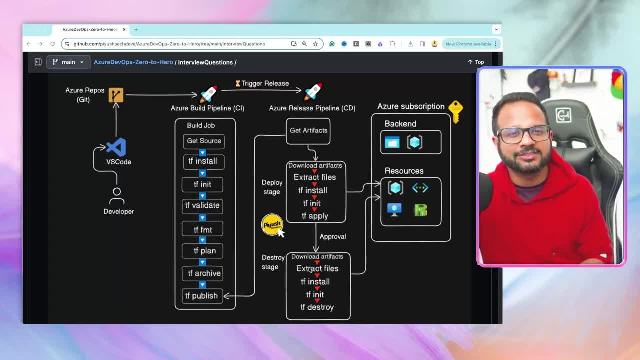 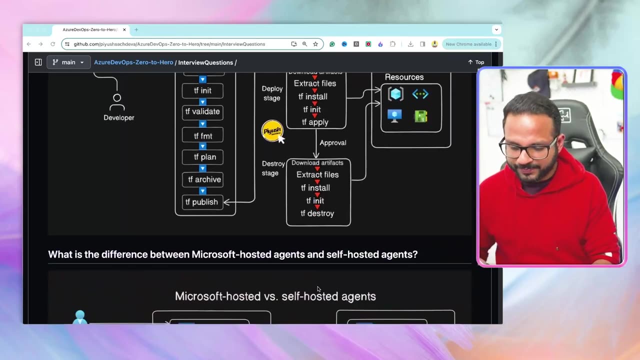 will be destroyed. So this will make sure that once your testing is done, once you've done all the validation and you have all the- you know- checklist items, you can destroy the resources and you can save the cost And, like you, can follow all the best practices. Okay, so now the next question could be: what is 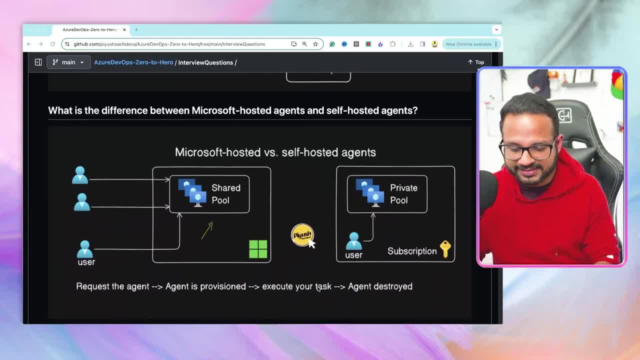 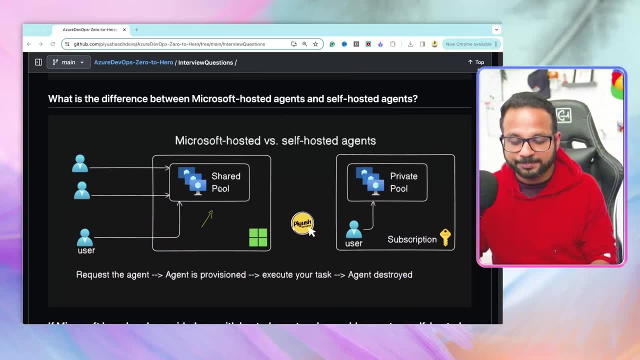 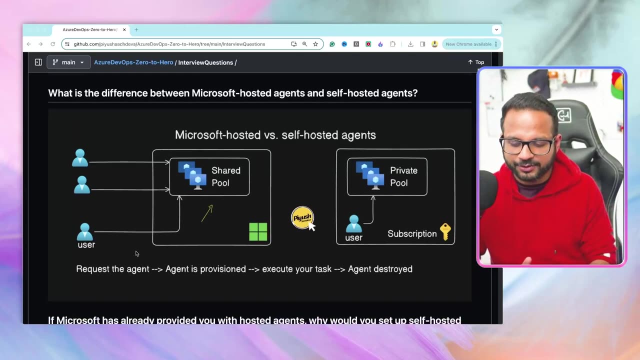 the difference between Microsoft hosted agent and self hosted agent. So you can try by explaining the difference. like, let's say, Microsoft hosted agents are part of the shared pool that's been shared among multiple users, among multiple organizations, And you know you request an agent whenever you trigger the pipeline And if you have specified 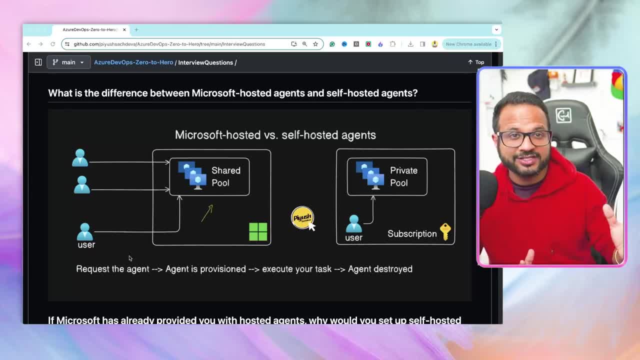 to use Microsoft hosted agent. the request will be sent to the agent from the shared pool. then, after a few seconds- you have to wait for a few seconds sometime- And then agent will be provisioned based on the availability And then it will execute your task and then it will be. 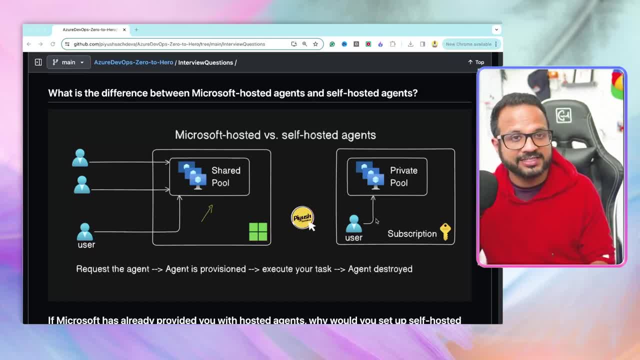 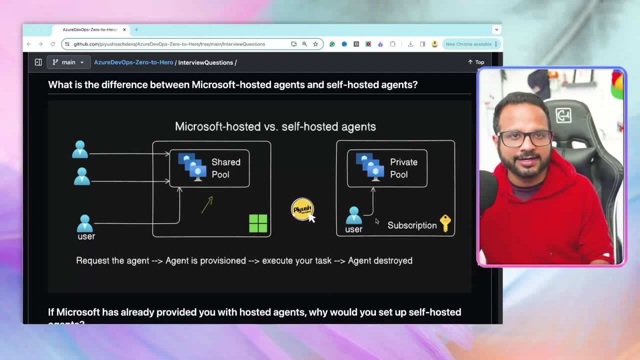 destroyed. But if you are using self hosted agents, it will be part of your own private pool that you have hosted right. it will be available all the time. you can install it as a part of your machine scale set and make it highly available, highly scalable and fault tolerant. so 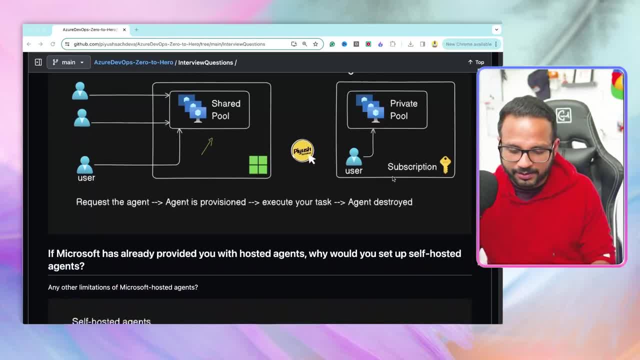 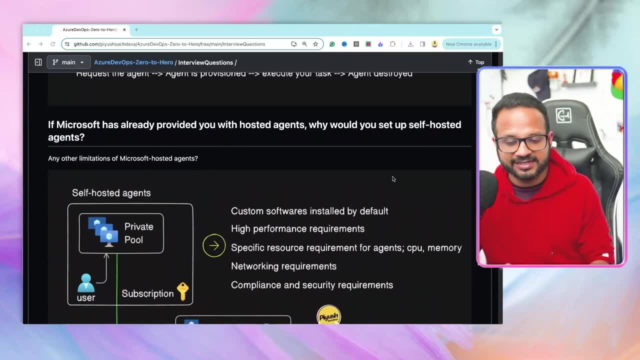 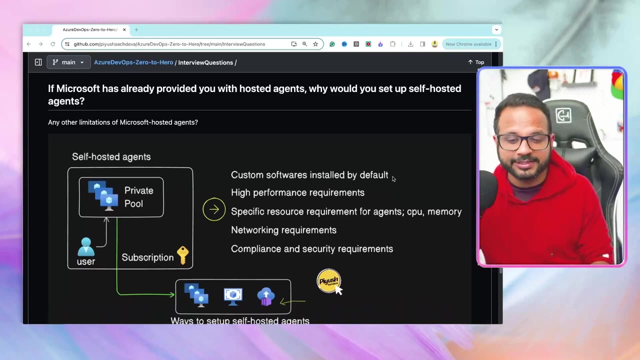 that it is available all the time. Now there will be a question like: if Microsoft has already provided you with the hosted agent, why would you go on and set up your own self hosted agent And what would be the benefit or what would be the use case of it? So few use cases that we 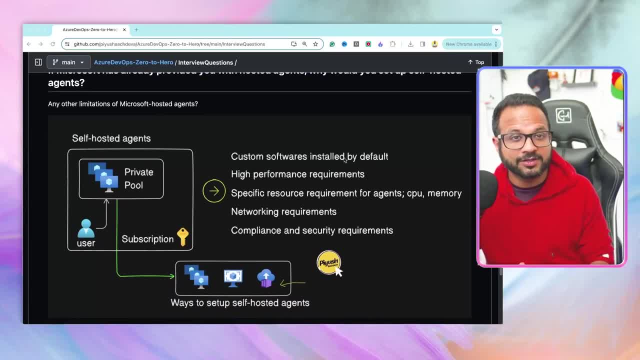 have just discussed. like you don't have to wait for the agent to become available, I'm sure that we will slowly be able to support the agent, But you do want to install yourself as a dedicated agent using an infrastructure that you are not responsible for. that you cannot. 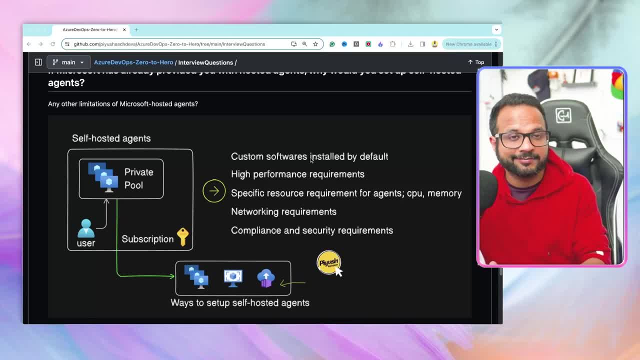 use as a dedicated agent. let's say, you just install a plugin And you will then have to redeploy the auto install. you're notissa. if that's the way you want to do it, You have to regulotry install it from the resource pool, right? So it will be fast. Then you can install your. 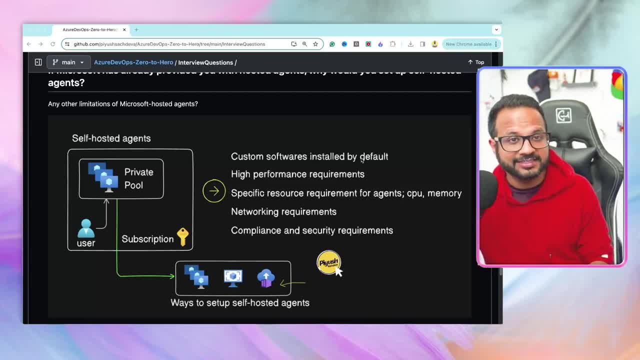 custom software by default, Because if you're using Microsoft hosted agent, you have to install. Let's say, if you were using Terraform, Yes, Yes, Yes, Yes, Yes, Yes, Yes, you can have a terraform, cli, azure, cli, anything that you want. you can pre-package that inside. 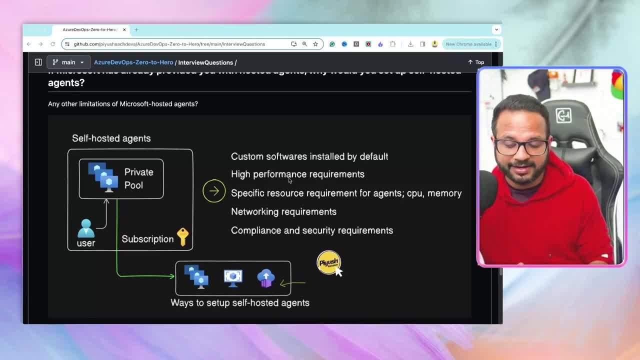 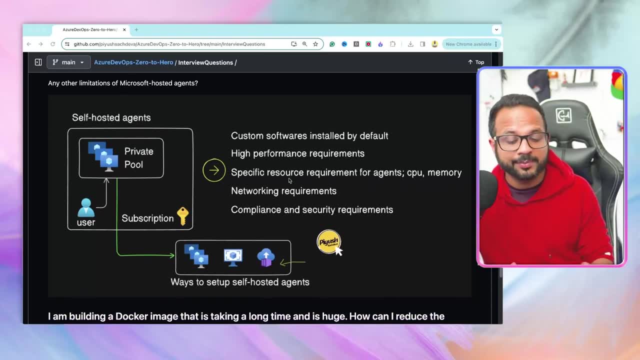 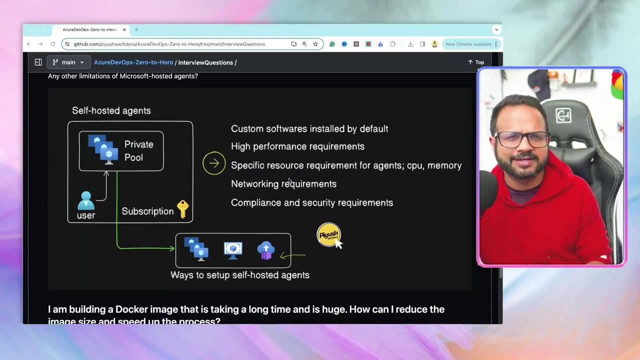 that. so that is one of the important requirement and you could have a high performance requirement for your build agent. you could specify more cpu, more memory, more storage for your agent so that you are not restricted with the default options by microsoft. you could have some specific network. 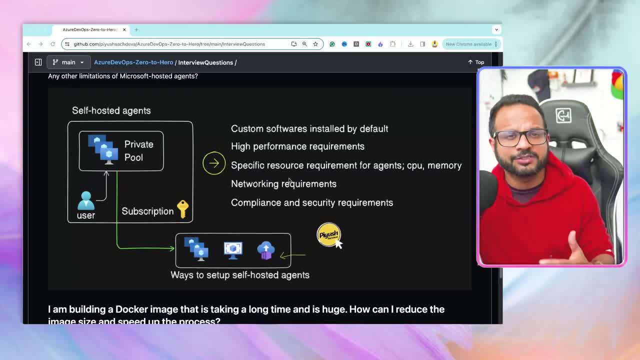 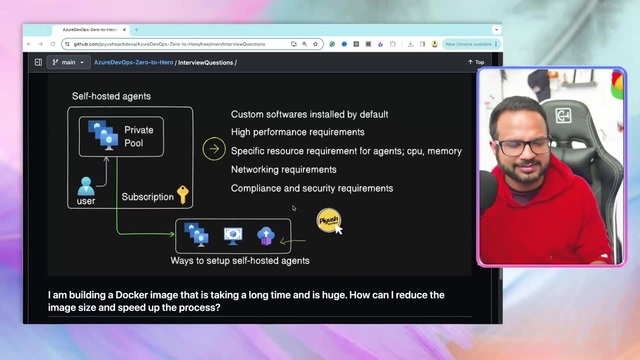 requirements like your build should not be traversed through the public internet, which it does, by the way, in case of microsoft hosted agent. if you are using self-hosted agent, it will be there within your azure subscription, within your secure environment, and you could have certain compliance and security requirements as well, so self-hosted agent is a good choice for production. 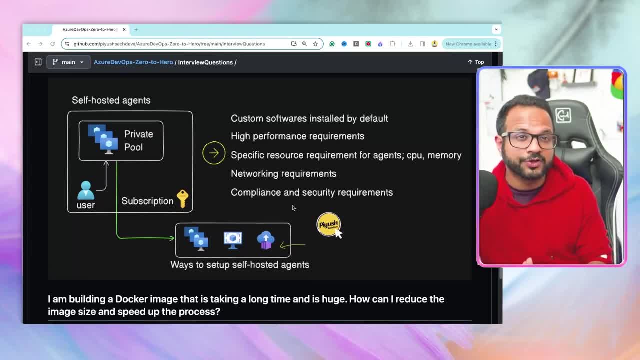 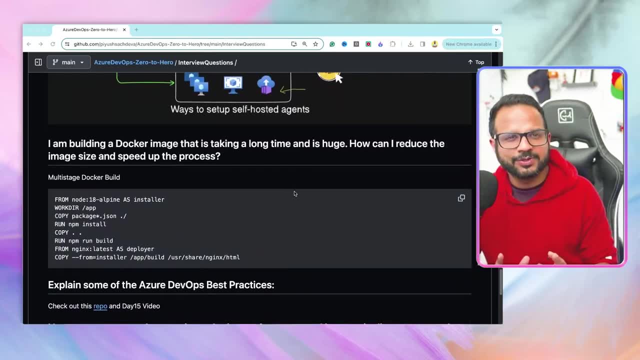 workload and it will give you more control over your agent and workload running on it. the next question could be: it is not specific to azure devops, but i thought of adding it because we have covered docker kubernetes as well in this series, so it could be like i'm building a docker. 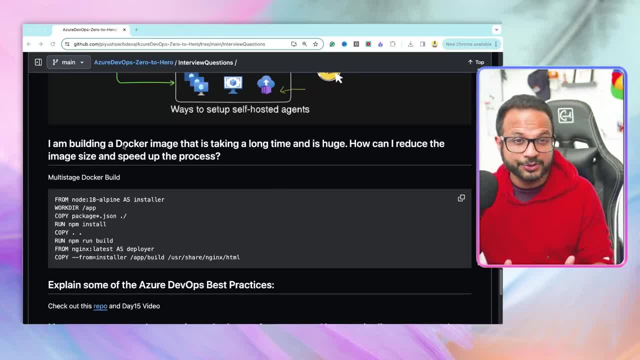 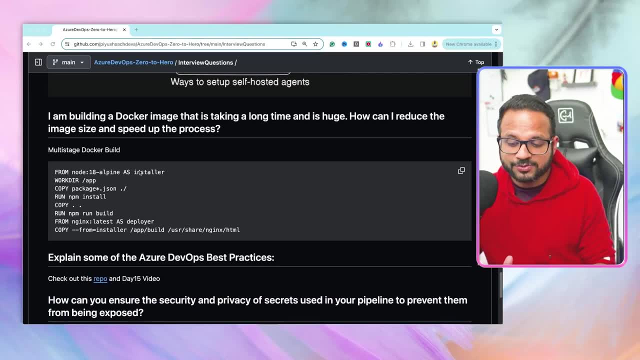 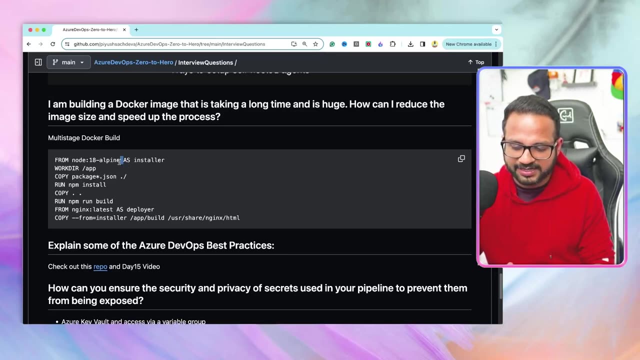 image and that is taking a long time and it is huge in size. how can i reduce the image size and speed up the process? the answer to that would be by using multi-stage docker build right. what it does is, let's say, we have two different stages. one is the first line, from node 18, alpine, as installer. 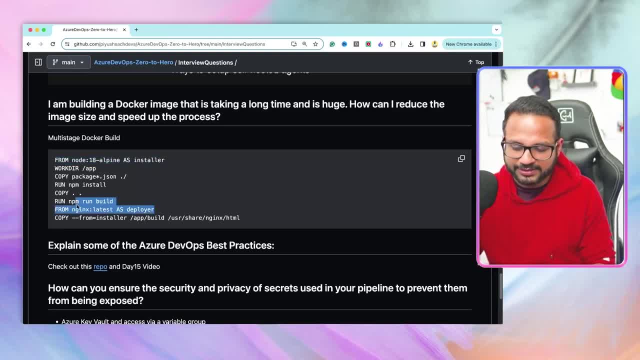 the second stage is deployer. so what we will do is we'll do everything on this base image, like with: we took node 18 alpine image as the base image and it has an installer stage in that we have a work directory and then we copied. 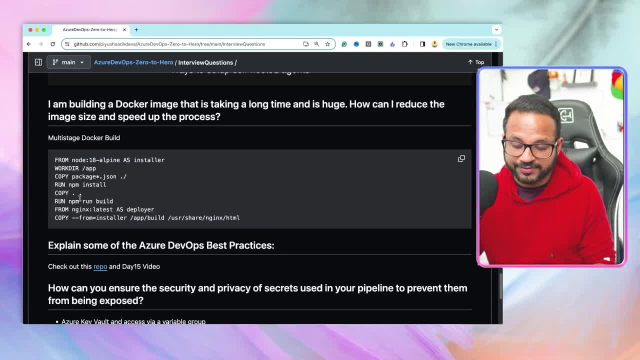 packagejson to the directory. we run npm install, we copied everything and then we run npm build. now we only need build folder for the application to become available. but over here we have the node modules folder with all the binaries and libraries which we don't want, and it will be. 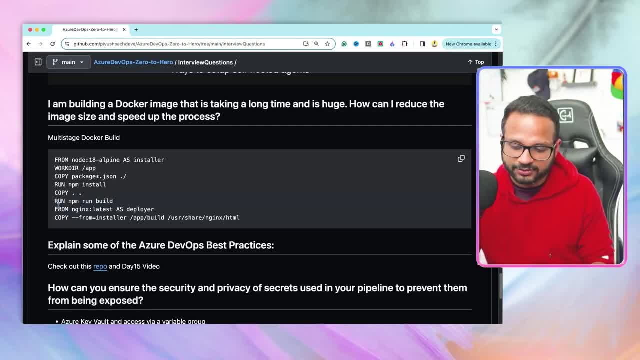 huge in size. it will just slow up the process. so that is why we created one more stage, which is taking nginx as the base image and from the installer stage, copy from installer. we are copying the build folder to this particular image, so now we will only have the build folder as part. 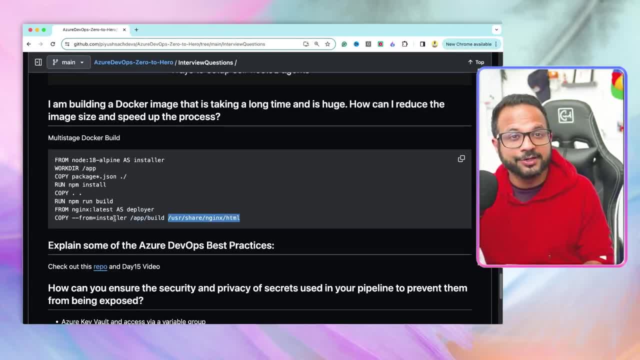 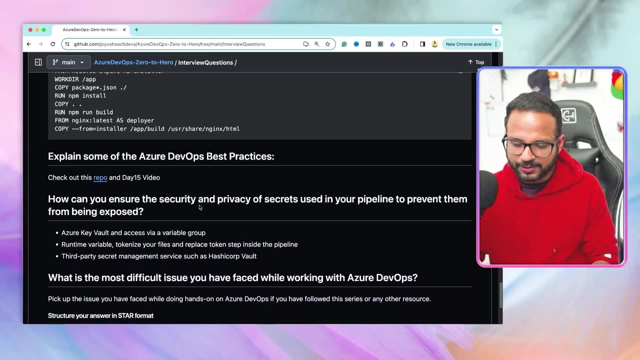 of our docker image, so this will reduce their image size drastically and it will significantly improve the performance of the build creation. so multi-stage build is one of the production best practices as well, so make sure to understand this. now explain some of the azure devops best. 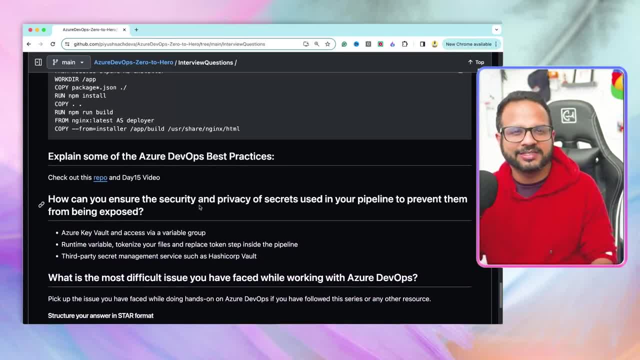 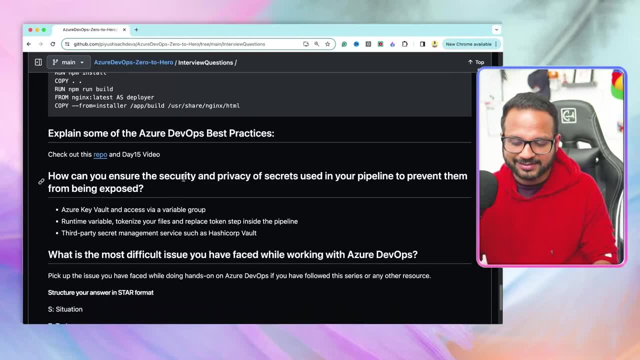 practices in terms of security, authentication, authorization and, you know, performance, reliability, operational excellence and so on. so for that, the build folder will be taking nginx as the base image and from the installer stage copy from there is an end-to-end dedicated video. so check out this repo or day 15 video. it will have all. 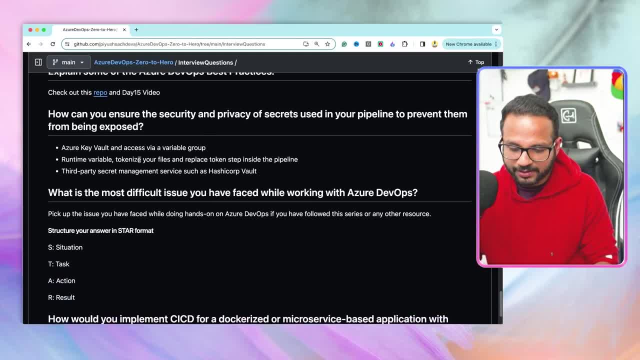 the details right. we have covered it recently. how can you ensure the security and privacy of secret used in your pipeline to prevent them from being exposed? like you should never upload your secrets into pipeline, doesn't matter if you are using uh it on production or you know a personal. 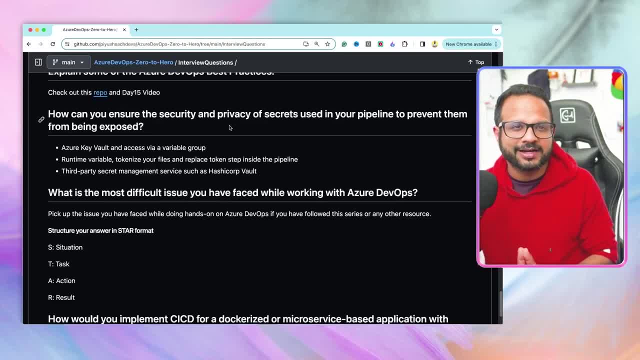 project, or if you are doing it for learning purpose, you should never upload it on the repository. so what options do we have? the first one is azure keyword. so you create an azure keyword, you know you grant your service principal access to that keyword to get the secrets. 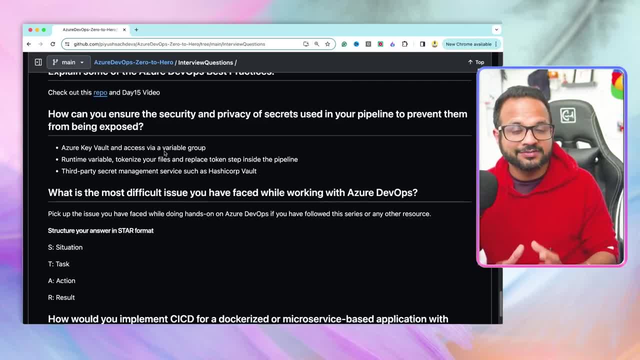 from with the help of pipeline and using a service connection, you get the access to it right with the help of pipeline variable if you are accessing it from the pipeline. the second option is to use a runtime variable. we have also, uh, used this one of the video demo right, so have a look at that. 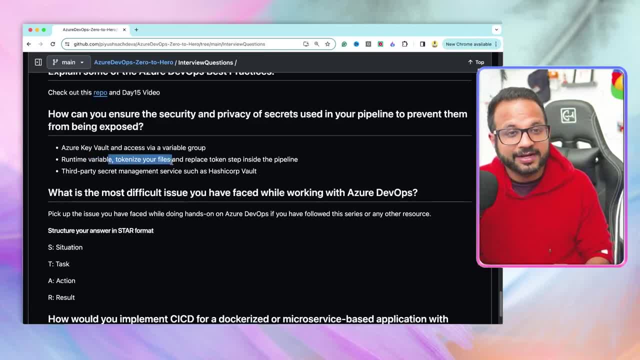 and runtime variable, and then you tokenize your file and then you replace your token with the help of a step inside the pipeline. and the third option is you can use a third party secret management service, such as hashicorp vault. so i am aware of these three there could be. 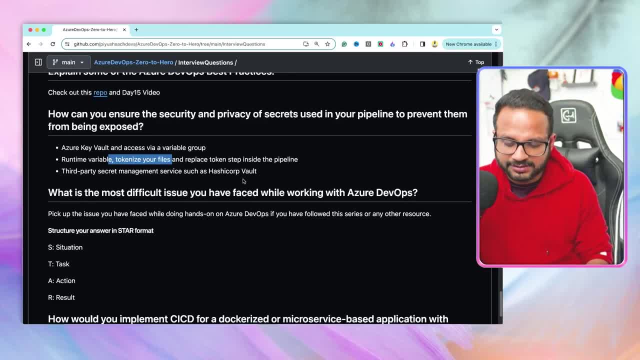 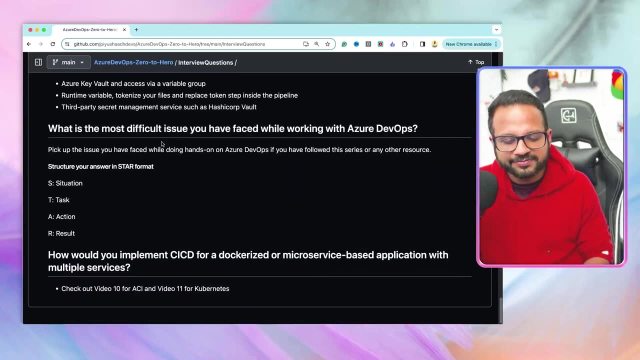 many more right, but these three are the standard ones and, out of these, i should say, i should say the most common and most secure when it comes to interacting with azure devops. right then, what is the most difficult issue you have ever faced while working with azure devops? if you have done the 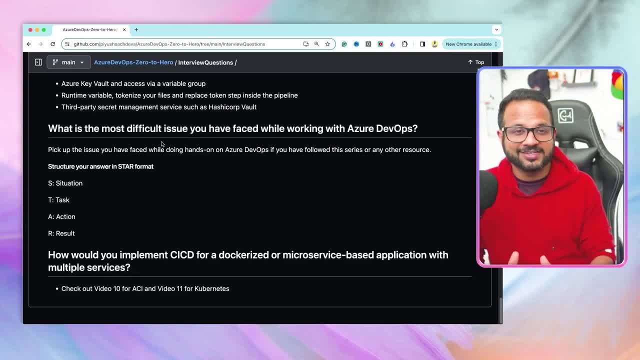 hands-on while following this playlist or any playlist or anything you know. if you have done the hands-on, you might have faced a lot of issues. if you have not faced a lot of issue, that means you have not done it enough. you you have not done it deep enough. 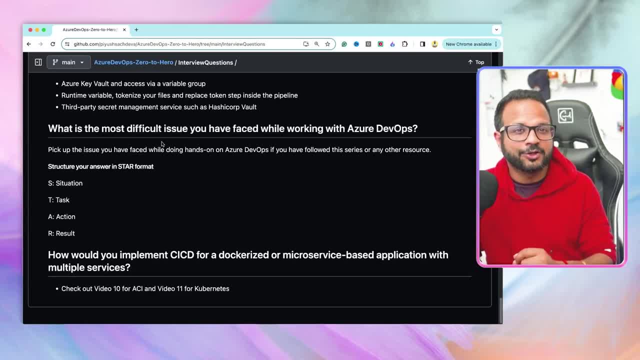 so make sure you do that, and if you have faced the issue, so document it somewhere in your notepad, in somewhere that is easy for you to remember or to revise later on, and then, when this question has been asked, you can structure your answer in star format. star format is you start with telling. 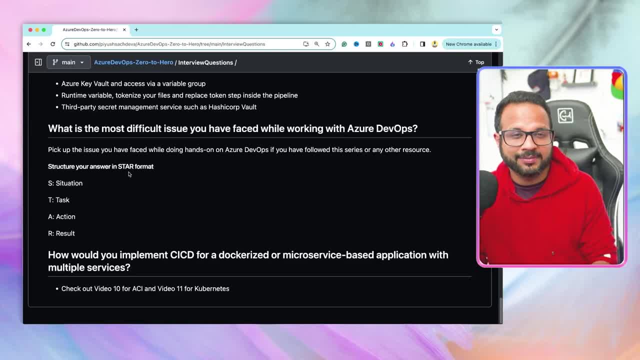 the situation- okay, i was learning or i was implementing something and i was facing this issue. then implement the task like: what exactly were you doing? then action, like when you face the issue: which all troubleshooting steps did you take? right and list down all the steps and what happened eventually and what was the result. 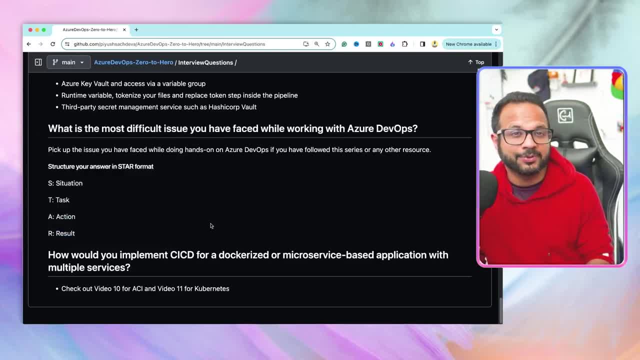 like: how did you resolve the issue? you seek help. you took the community support or you tried. after a few days you enable debug logs. you ssh into the server and you check the diagnostic logs. you check from the kudu console if your files were deployed. you check all the pipeline logs. you 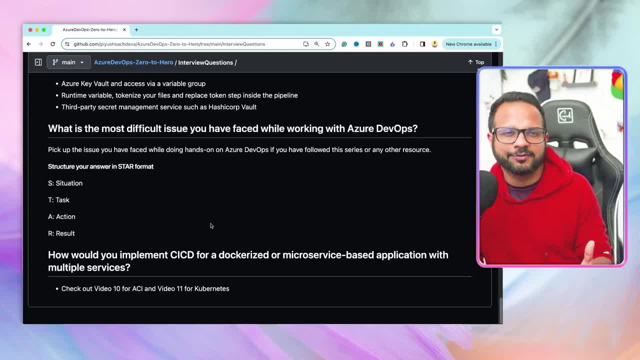 deployed it manually and there could be many more steps that you would have taken. so define all those steps and how it was resolved then. how would you implement cicd for a dockerized or micro service based application with multiple services? so these were part of video number 10, in which we 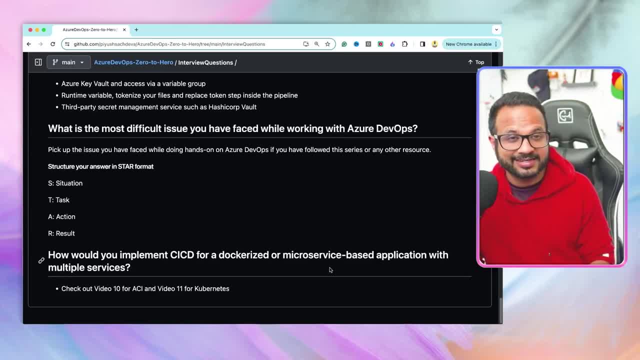 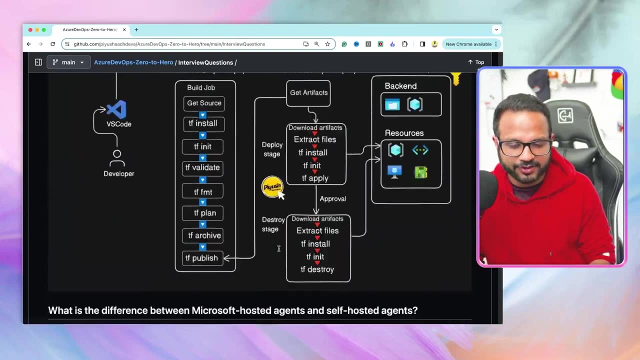 have dockerized an application and deployed it to azure container instances, and video number 11, in which we deployed it to aks as your kubernetes service, so you can have a look at that- and you might already have done that then it's good. so this is the repository that i wanted you to have. 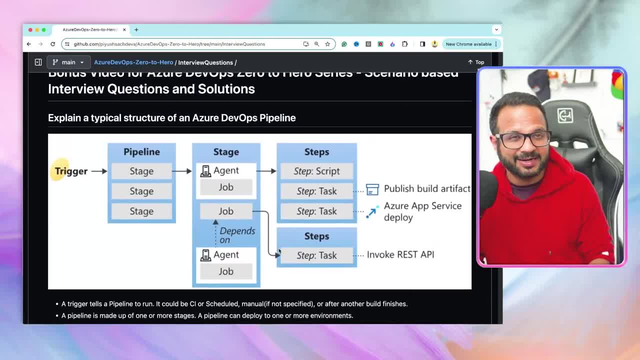 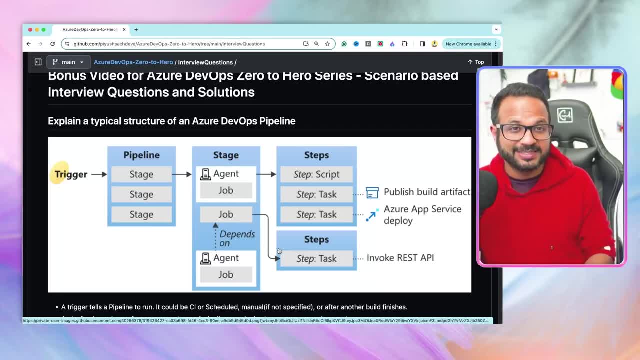 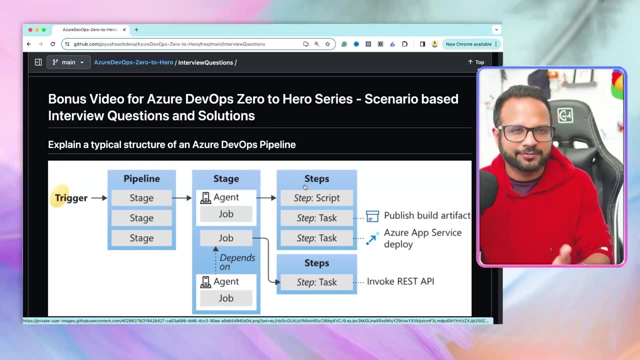 a look along with me. now that we have seen it, i'll keep it updated. i will whatever i remember or whatever issue i face, or if you also face the issue, please start a pull request and i will review it. i will definitely add that in the interview questions or any other folder, if